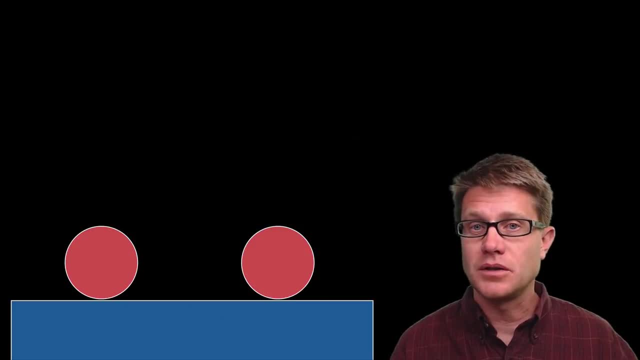 second one, And so a good question might be: which has experienced the most dramatic change in momentum? That is kind of a trick question, Since they both have the same mass and the same velocity and at the end they are at rest, they have experienced the same change in momentum. 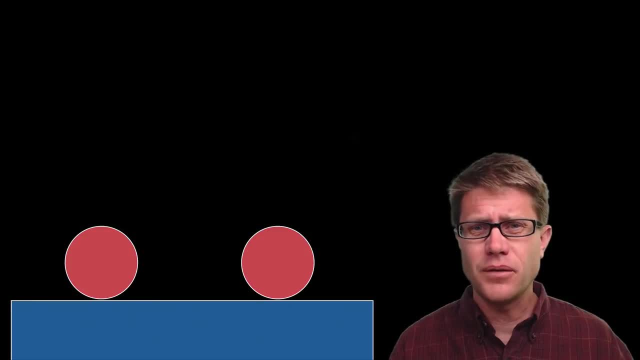 Therefore, their impulse is the same, And so what is different in these two spheres as they fall to the table? Well, it is the time over which they interact with each other. With the table itself, The one on the right is really slowing down over a longer period. 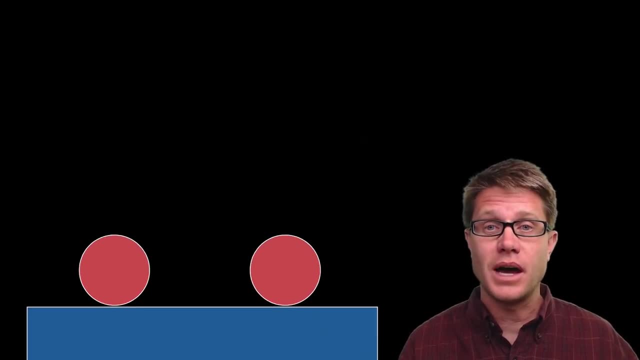 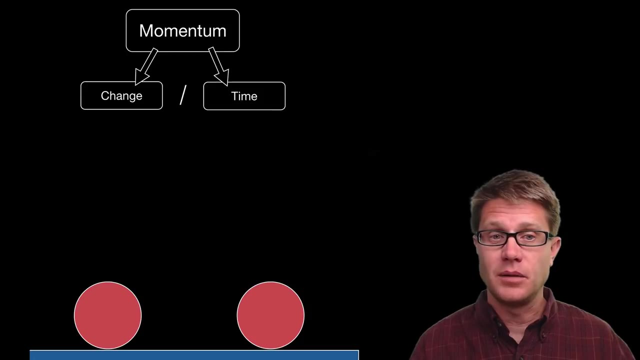 of time, And that means it is applying less force to that table, And so momentum will change over time. And so, if we have these two spheres, the momentum is going to be the same between each of those. The impulse is also going to be the same. What is the impulse? 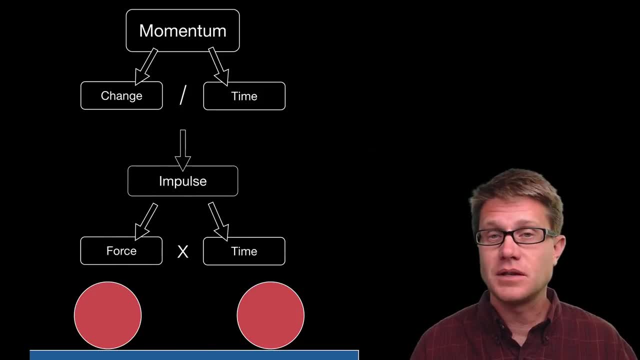 It is simply multiplying the force of an object times the time of that object, And these are equivalent. The change in momentum and the impulse are exactly the same. So the momentum is exactly the same thing. And so what is different in these two spheres? Well, in this. 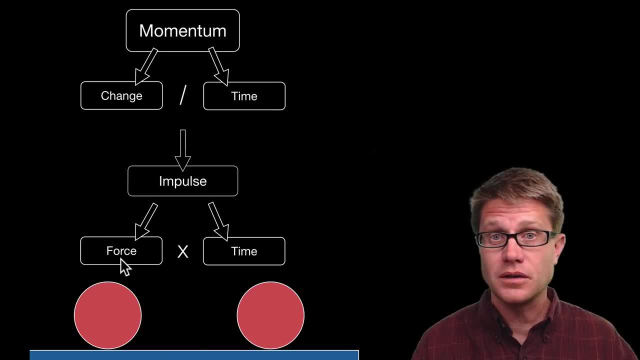 sphere. right here, what we are getting is a really large force over a short period of time, And in this one, we are getting a really short or a small force over a long period of time, And that fact is so important that it could literally save your life. Cars have 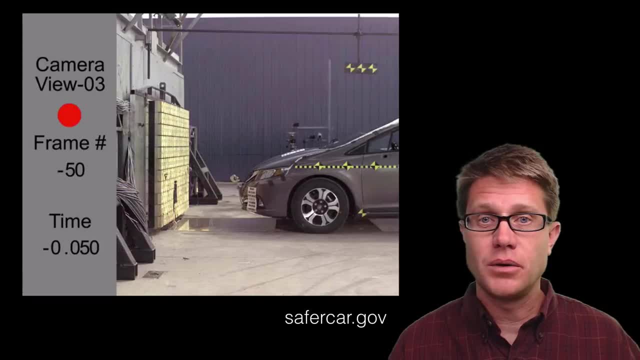 gotten safer and safer over time, And so this is a safety video. If we were to crash a 57 Chevy- an old car- into a wall at 35 miles an hour, the person inside would really be hurt, Because it is going to come to a stop almost instantaneously. But watch what happens. 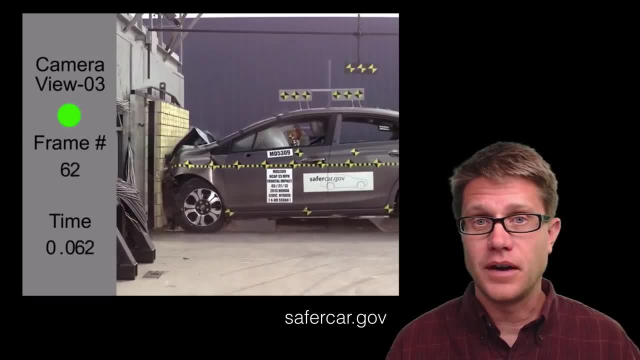 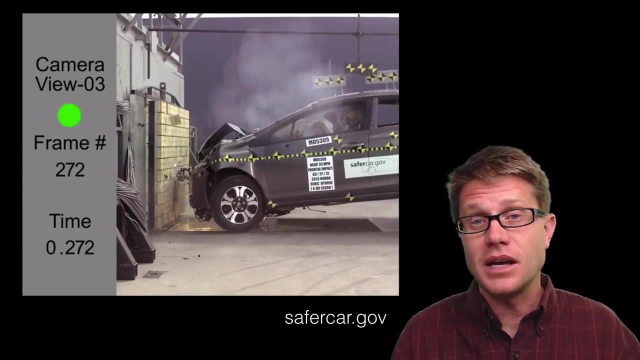 when this Honda Civic is driven into a wall at 35 miles an hour, Again, it is slowed down, But watch how long it takes for that car to come to rest, And so it is like that squishy ball. It is taking a longer period of time for it to change its momentum, And so we are. 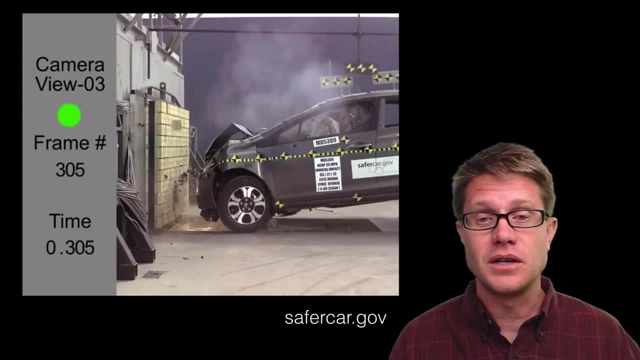 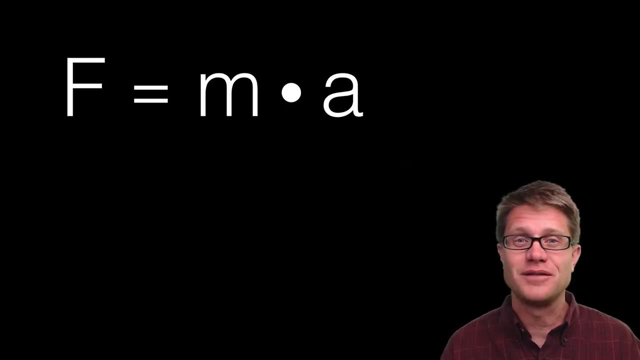 decreasing the force experienced by both the car and the person inside the car, And so to figure out how these two are related, it is really simple, And it begins, like every thing in physics, with Newton's second law, which is force equal to mass times: acceleration. 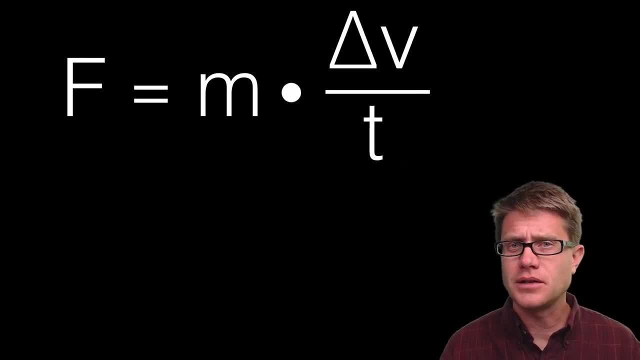 But let's break down acceleration, which is simply going to be the change in velocity over time. Now I am going to take both sides of this equation and I am going to multiply them times, time, And so if I do that, what do I get? The two subjects of this video. 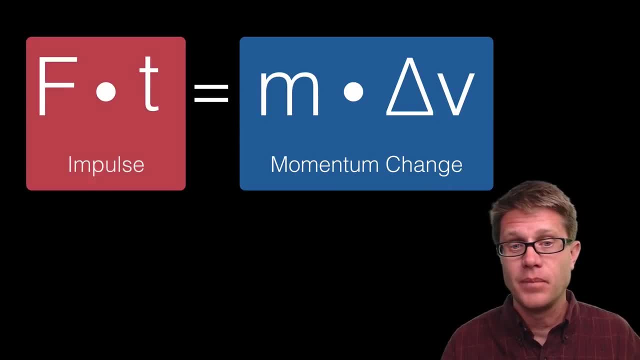 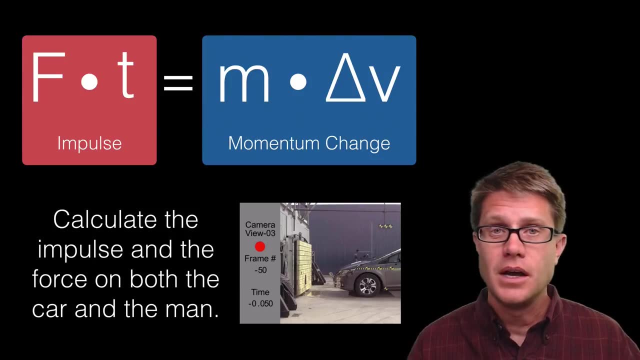 Momentum change, which is mass times the change in velocity. that is on the right, What is on the left. That is going to be the impulse And these are equivalent. So we can use it to solve really difficult problems Like: could you calculate the impulse and the force? 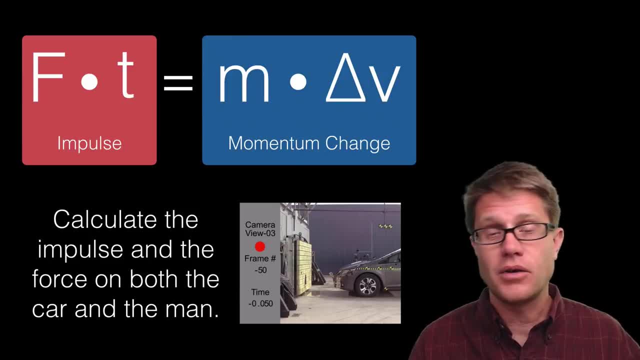 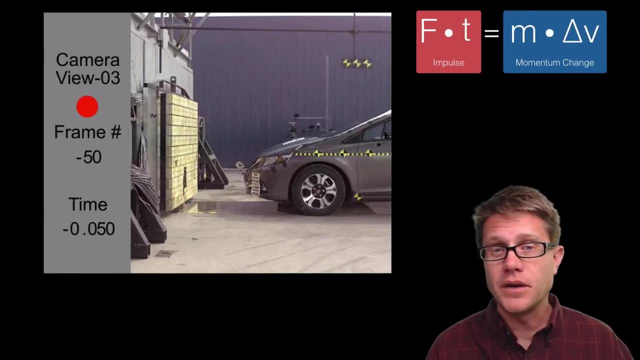 on both the car as it crashes into the wall and then the crash test dummy on the inside of the wall. Well, you will be able to, and we will work through a few problems like that, And so if you want to figure out what we need to solve a problem like that, it is all given. 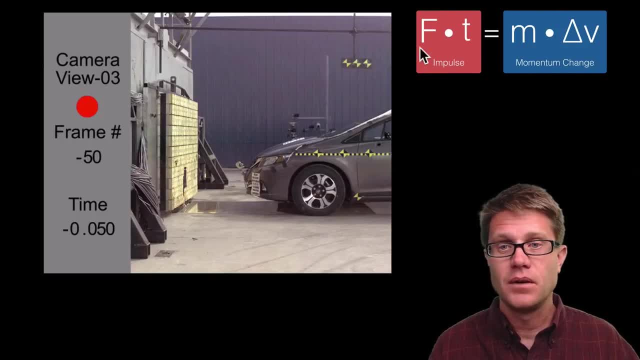 in the equations up here. Mass times change in velocity, Force, times, time. But we are just watching a video here, So you do not see any force in the video, And so we are going to have to solve for that in a little bit of time. 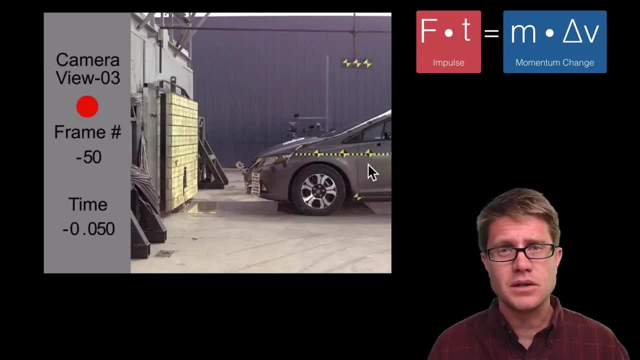 And so what would be the first things that we could figure out? Well, we have got to figure out the mass, And so I could just give you the mass. The mass of this car, which is a 2013 Honda Civic Hybrid, is 1301 kilograms, And the mass of the person inside the car. 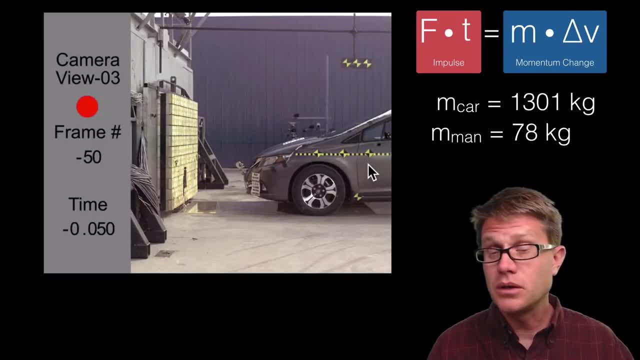 is around 78 kilograms. What else could I tell you? Well, we know. this car is going at 35 miles an hour, And at the end it is going to be going 0. And so we could see a change in velocity of 15.6 meters per second. What else do we have to figure out? Well, we have. 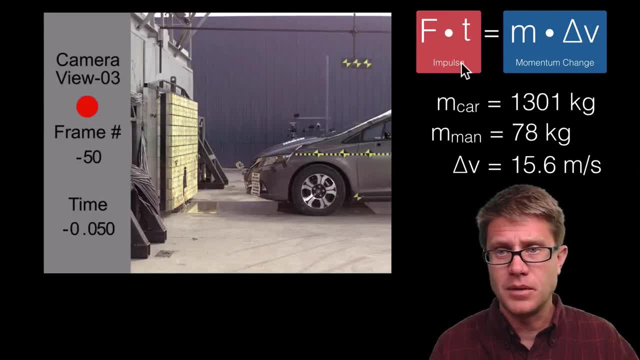 to figure out time. This information right here is enough for us to figure out the momentum change and the impulse, But if we want to get at the force being applied to the car and the crash test dummy, we also have to know the time, And so let us watch the video. 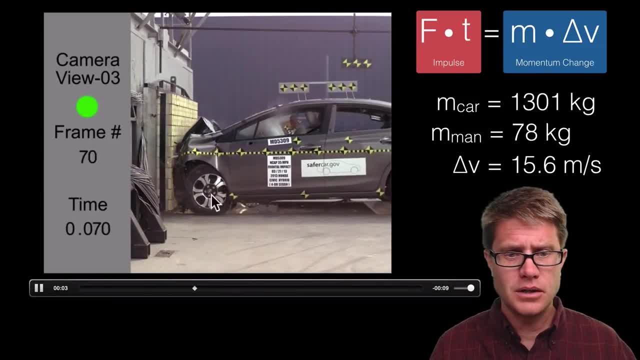 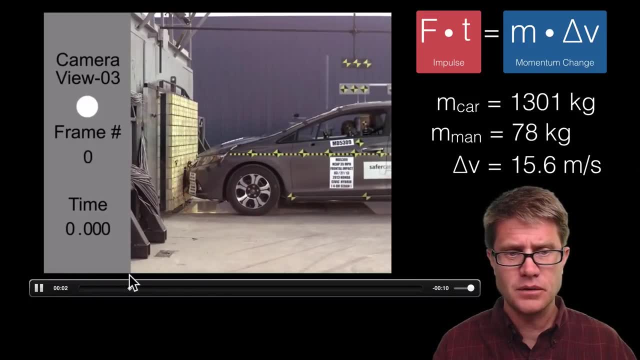 and let me show you how you can figure this out. So we have got the car crashing into the wall. I am going to grab the video right here And you can see here that right at this point, at time, 0, it is impacting the car And we have reset our time by 0. And we have 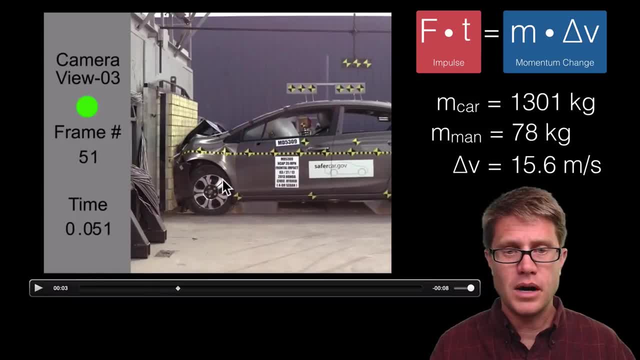 reset our time to 0. And so what I want you to do is: let's watch a section of the car, Let's watch this section of the car right here And let's see how long it takes for that car to come to rest. And so, again, we will go back to 0. So it is now at 0.. So we 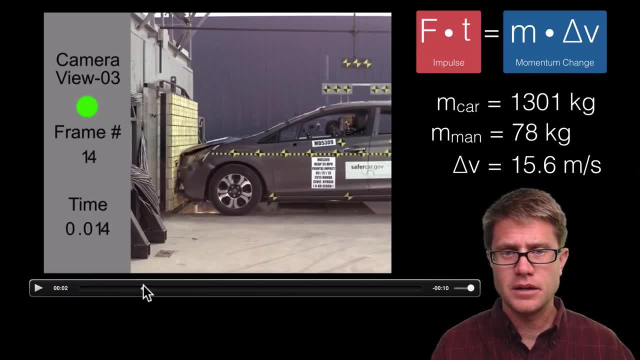 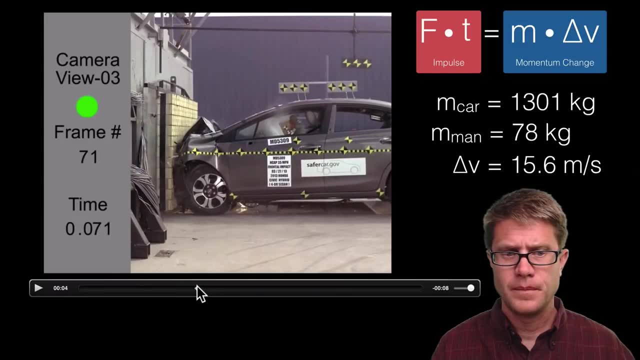 are at 0 here, And so just watch the car and figure out how long it takes for that car to completely come to rest. So let me keep moving. So right about there, So right about there, the car has stopped moving, And so we could say that that change in time is 0.072 seconds. I am getting that right. 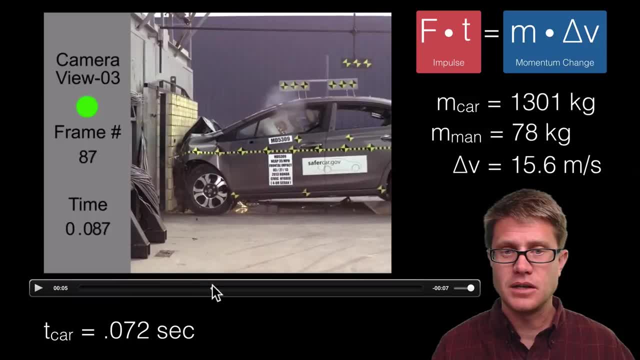 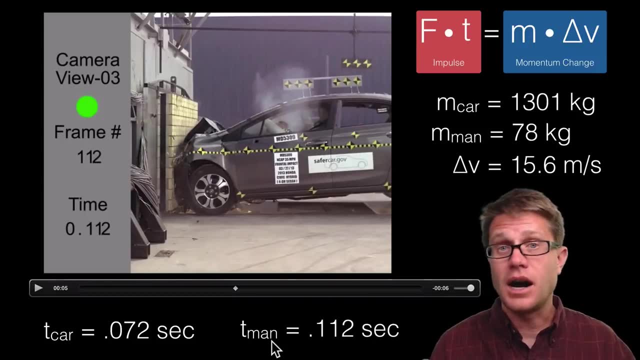 here, But if I keep playing the video, you will see that that person continues to move, They are still moving forward, And they do not come to a stop until around here, And so we could say their time of impulse is going to be 0.112 seconds, And so let me give you 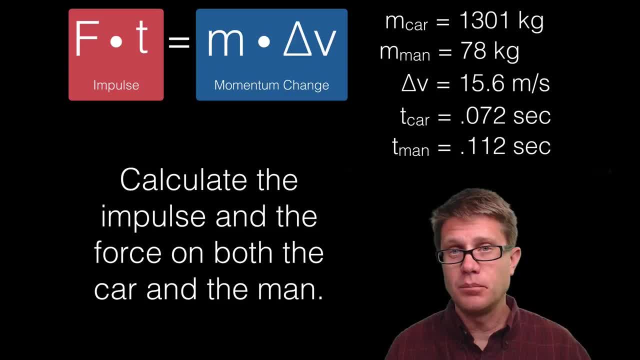 a simple problem. What I want you to figure out is calculate the impulse and the force being applied to both the car and the wall, And what we are going to do is we are going to have a three-dimensional process And we are going to have the man driving the car. 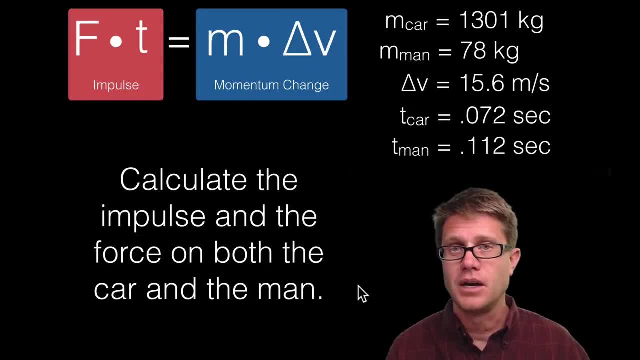 And this is going to be the car at the end of the car And this is going to be the man in the car, And so we are going to have this four-dimensional process, with the car and the man sitting within the car, And what I would encourage you to do is pause the video. 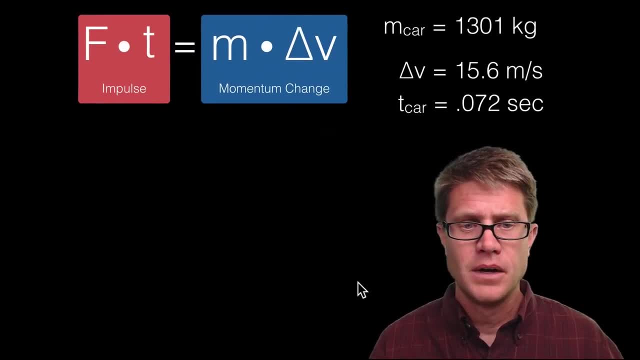 right here. You have everything you need right up here. I would grab a piece of paper and try to work this out Again. you are going to have four values when you are done: Impulse of the car, Force on the car. Impulse on the man. Force on the man. And so pause the video. 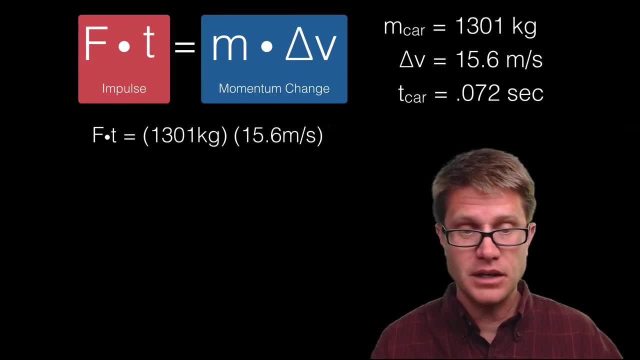 Try to work that out, But I am going to show you how to do it right now. And so what you equal to the mass times, the change in velocity. So I am simply putting in the mass, right here, of 1301 kilograms, The change in velocity of 15.6 meters per second. And so my impulse. 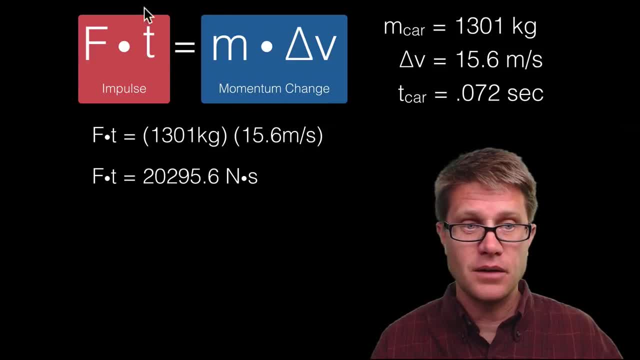 is going to be this: newtons per second. Now, how did I get that? Well, since it is a force times a time, it is going to be newtons times seconds. You can see here that this number has way too many significant digits, And so I could reduce that so that it has three significant 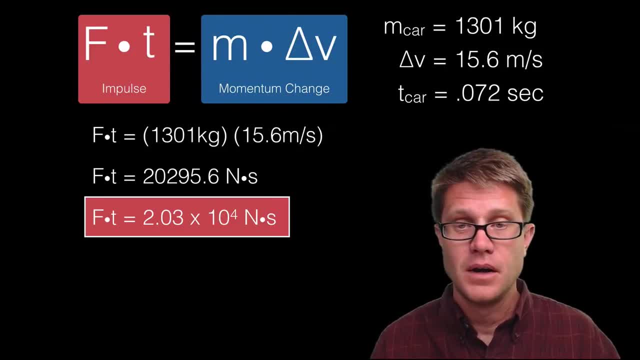 digits, And that is the answer of the impulse on that car. Now, how do we figure out the force being applied? Well, since I showed you the time- 0.072 seconds- if we want to figure out the impulse, all we do is simply divide by the time. So, if we divide it by the time, 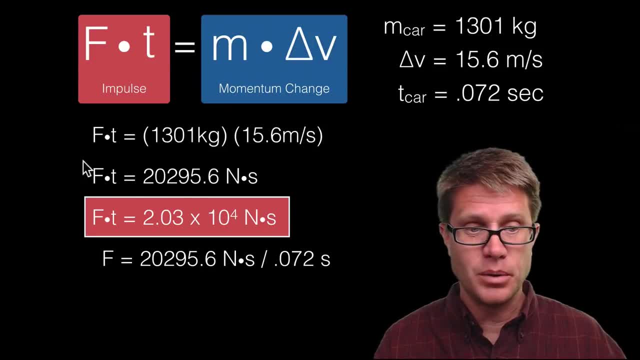 it is going to give us the force that is being applied. So I am going to take that impulse which is right here. I am going to include all those significant digits And then I am going to divide it by the time, which is 0.072 seconds, And it is going to give me a force. 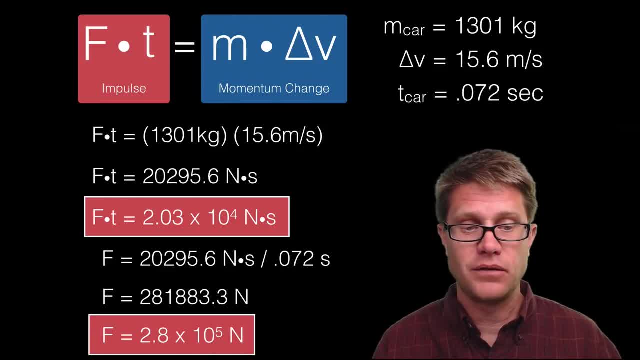 of that, And then again too many significant digits, I can figure out my force, which is only going to have two significant digits, And so it is going to be 2.8 times 10 to the 5th newtons. 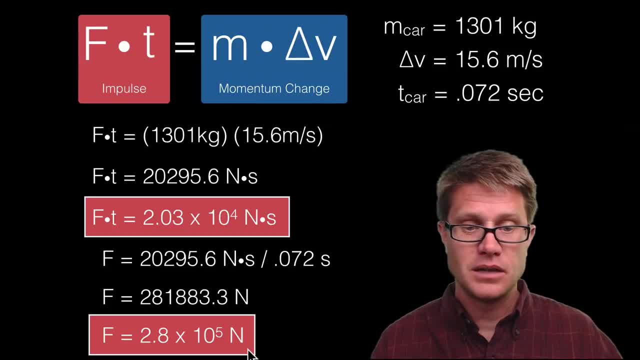 Why is that? Because 0.072 only has two significant digits, And so that is a massive force that is being applied to that car. But since the time is greater than it would be with an old car, it is actually going to be a much smaller force you would experience in a new age car. 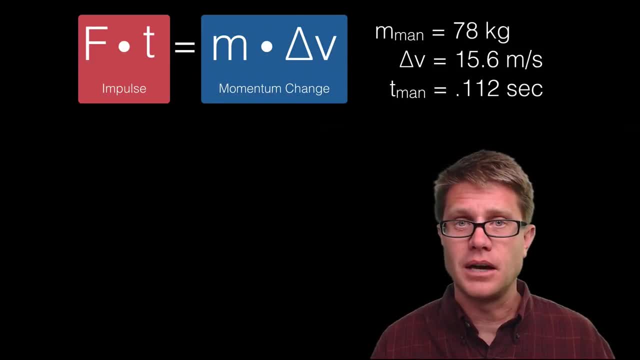 Let's say we were to look at the person inside it. How do we figure that out? again, Again, you could stop right now, And if you want to try to solve this one, you sure could. We are going to start with the impulse, which is simply: 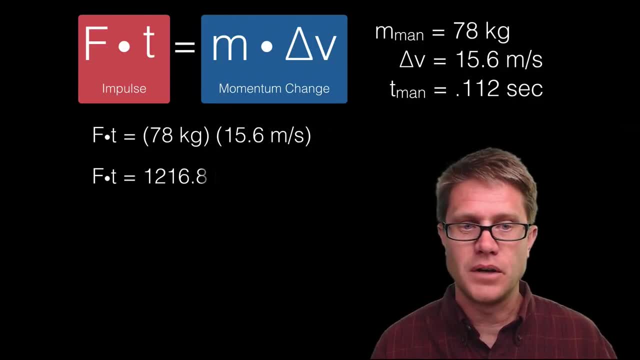 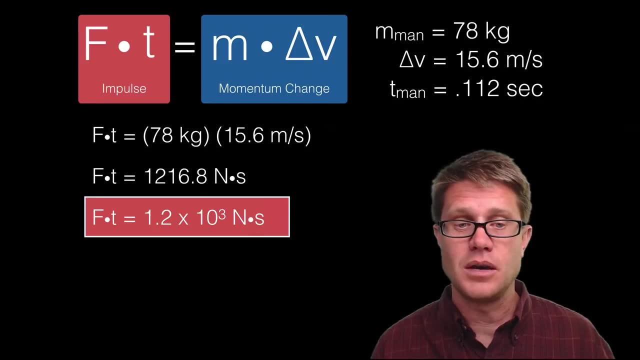 going to be the mass times, the change in velocity, And so I could figure it out like that: With significant digits it is going to be 1.2 times 10 to the 3rd newtons seconds. That is going to be the impulse. If I want to figure out the force, all I am going to do is going to 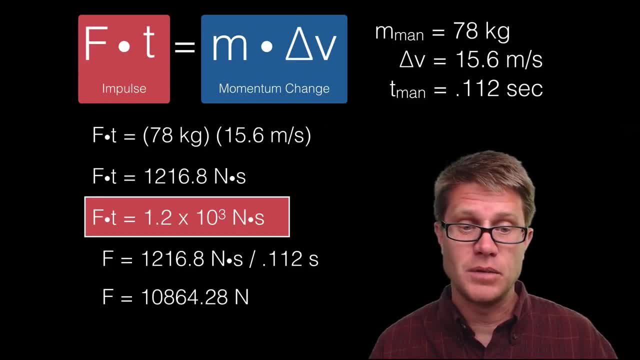 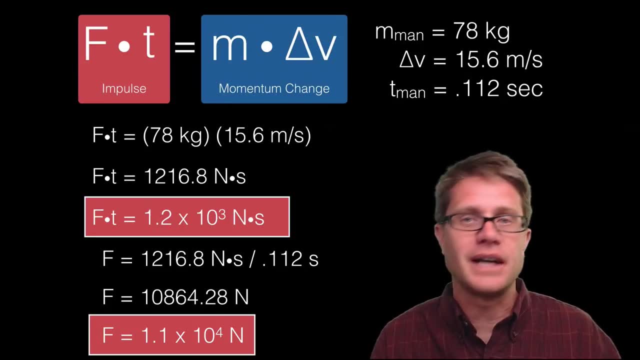 be to divide by the time, And so that is going to give me a value of around 1.1 times 10 to the 4th newtons, And so that is going to be the force that is applied to that person. Now, that is not a deadly force, And the reason why is that we have increased that amount. 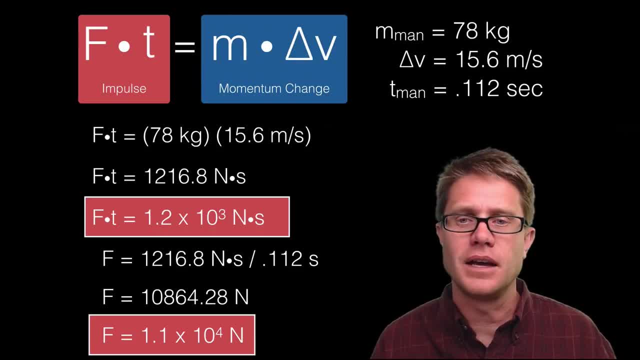 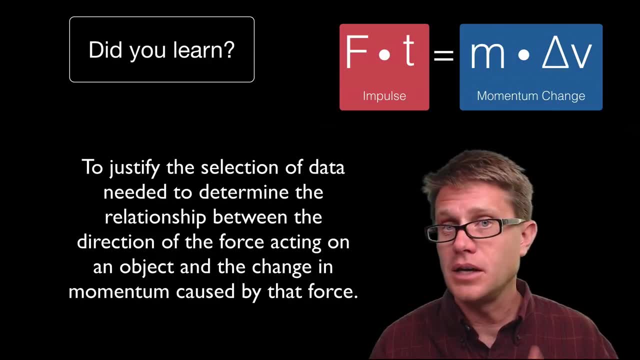 of time, Even though the momentum and the impulse stay the same. by increasing the time we can decrease the force, And so did you learn to justify the selection of data, if you want to figure out the impulse, or if you want to figure out the force, And then finally,